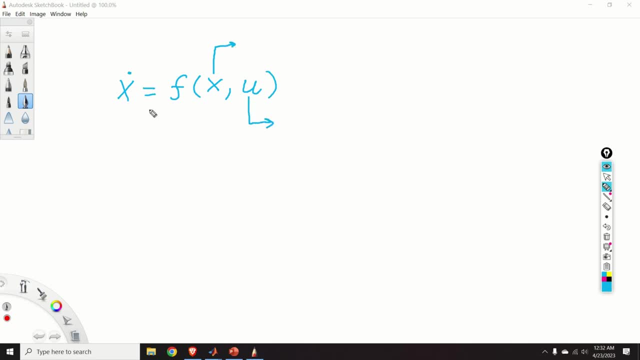 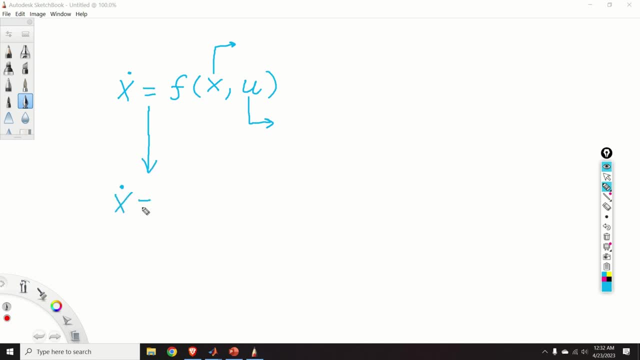 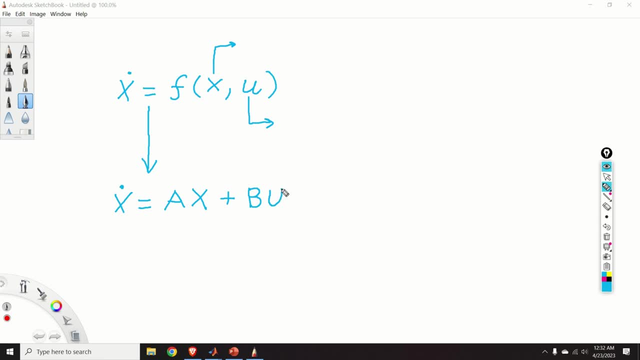 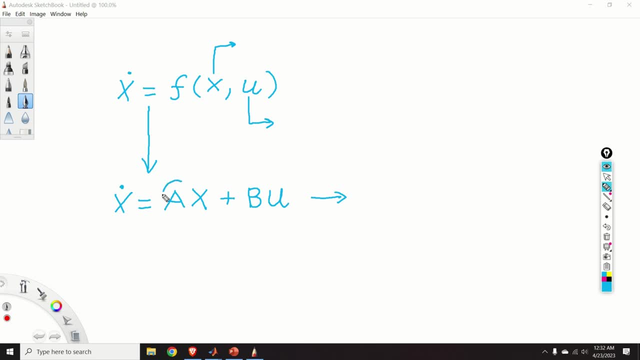 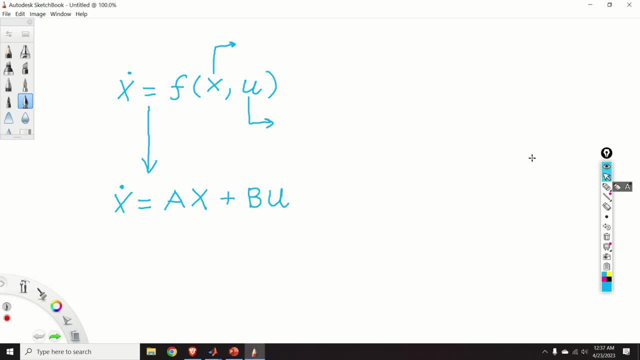 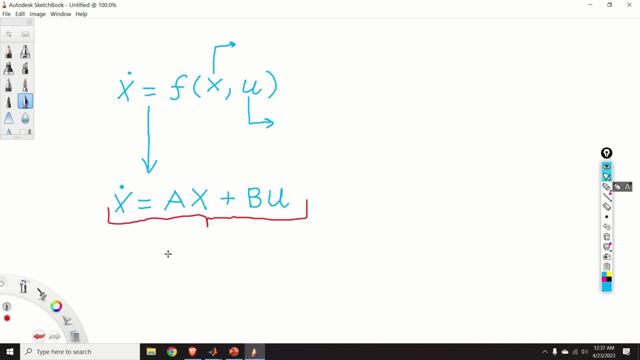 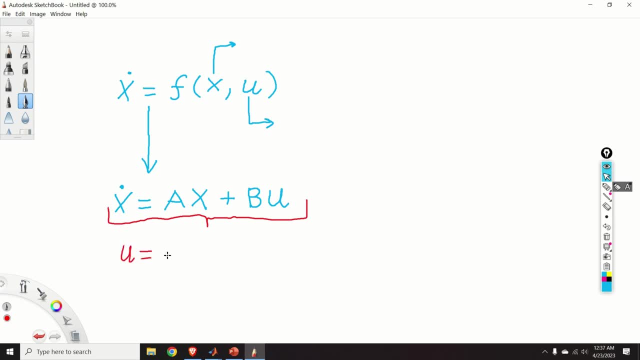 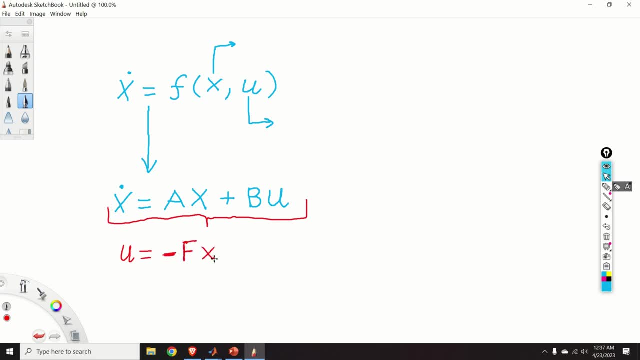 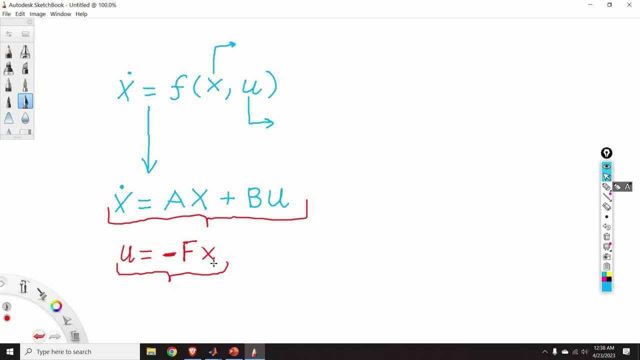 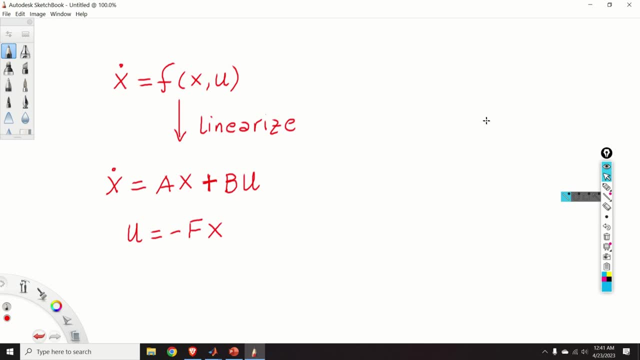 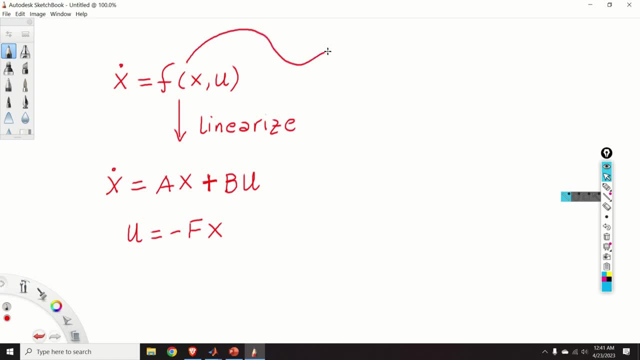 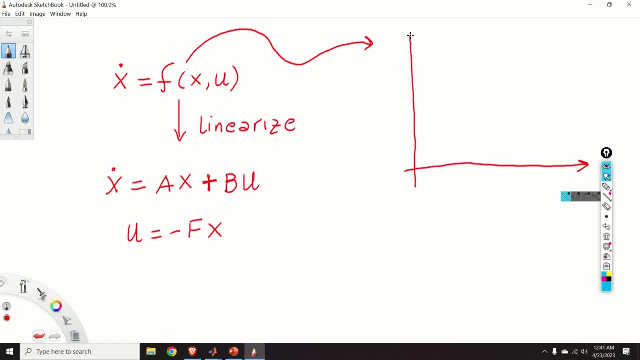 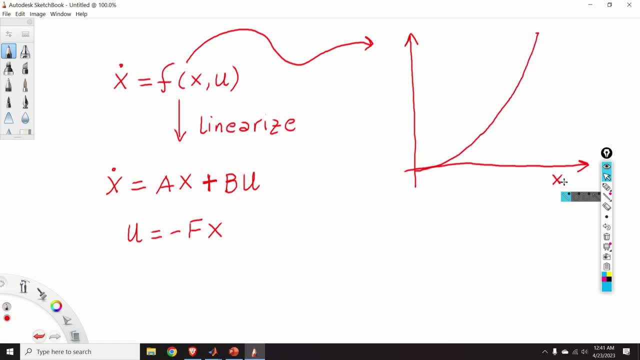 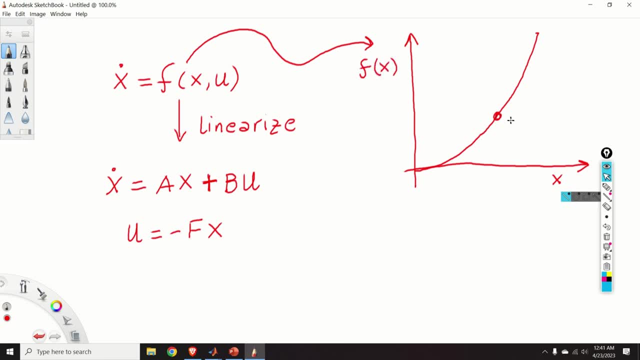 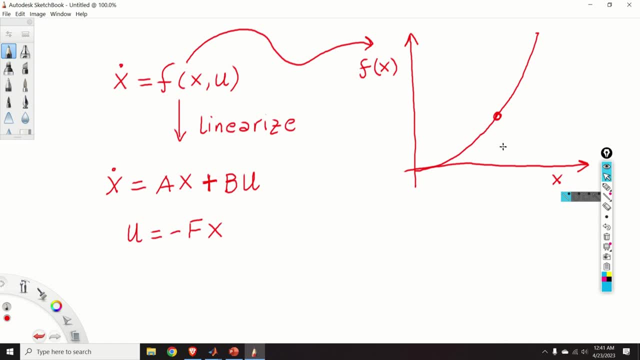 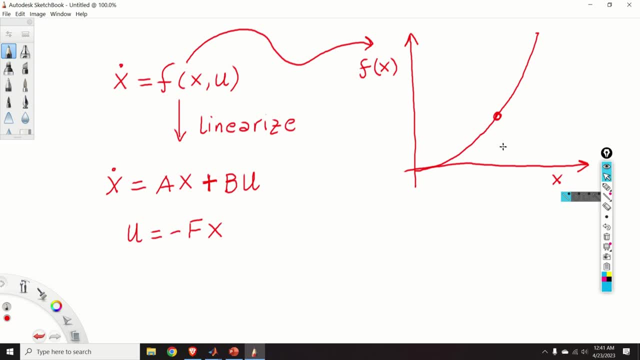 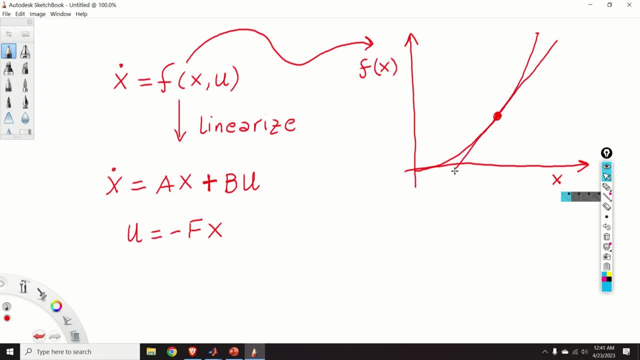 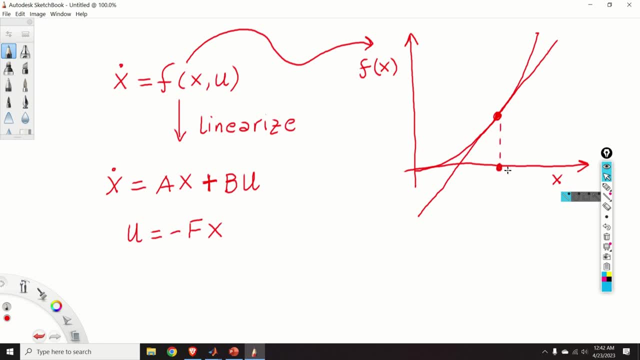 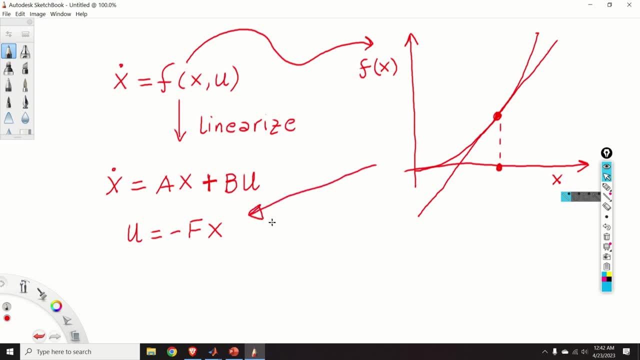 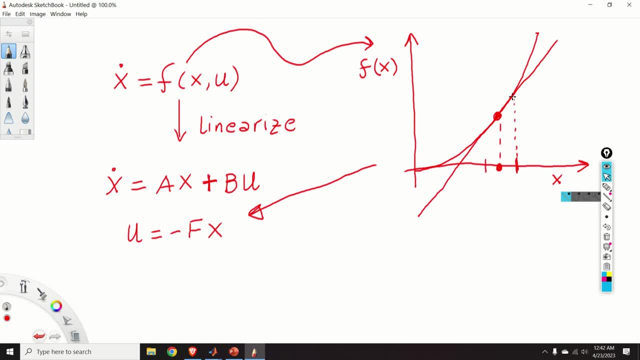 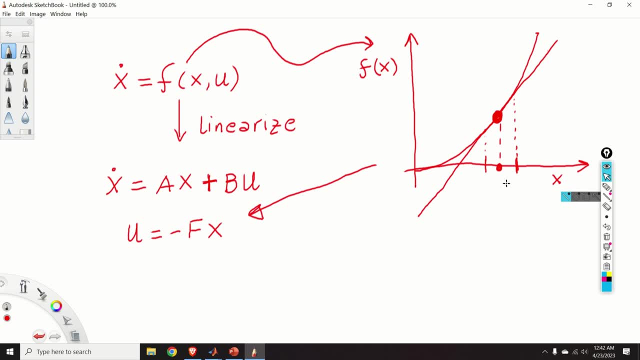 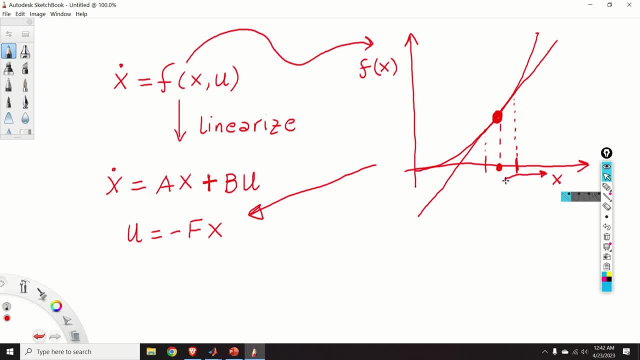 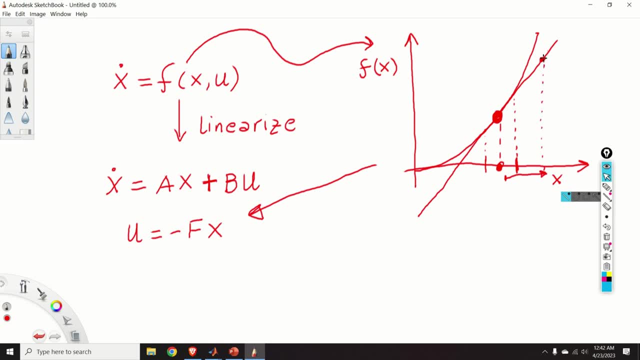 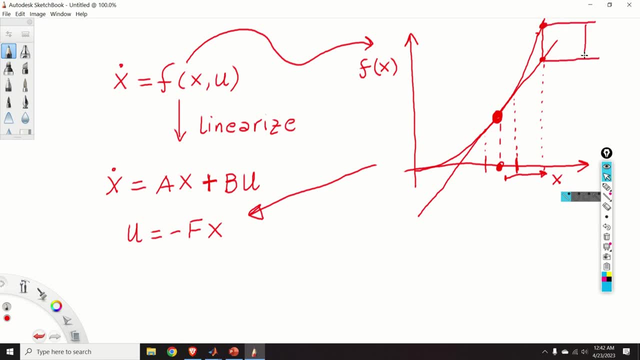 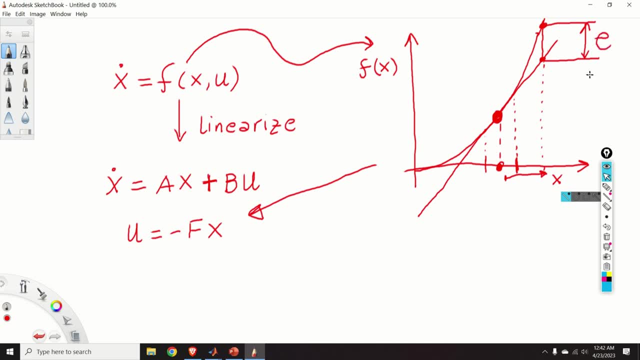 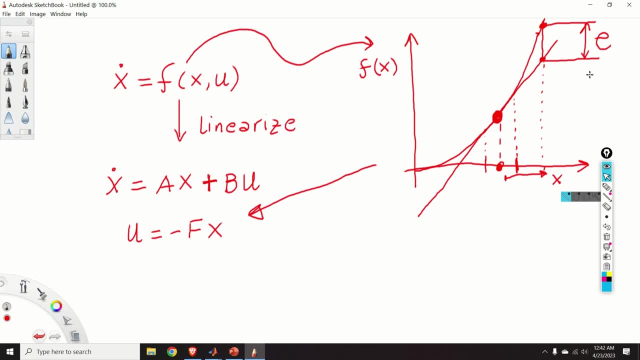 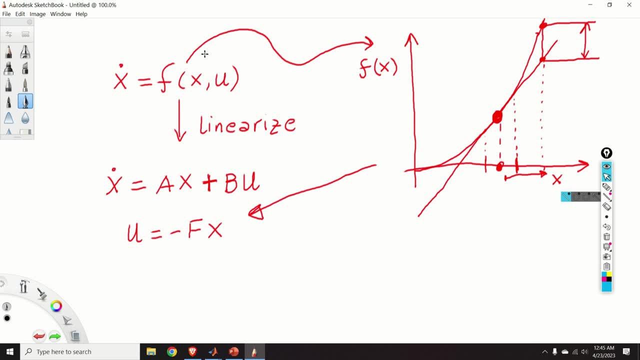 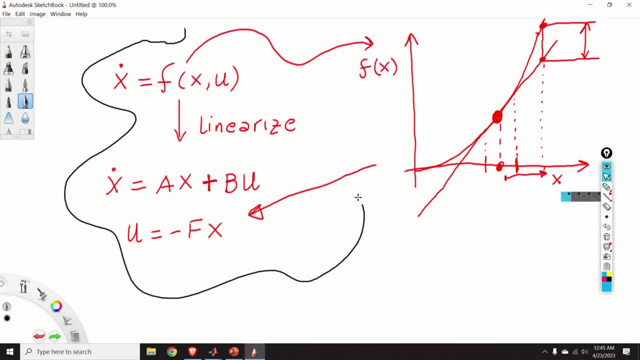 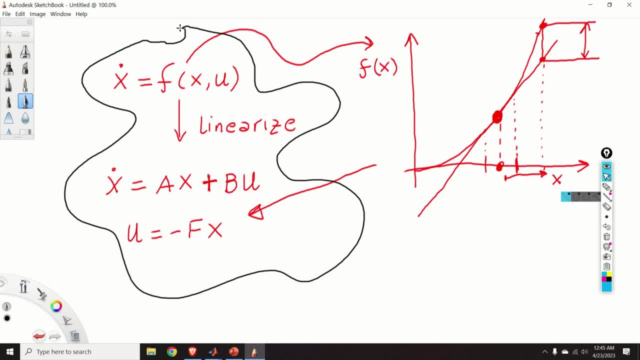 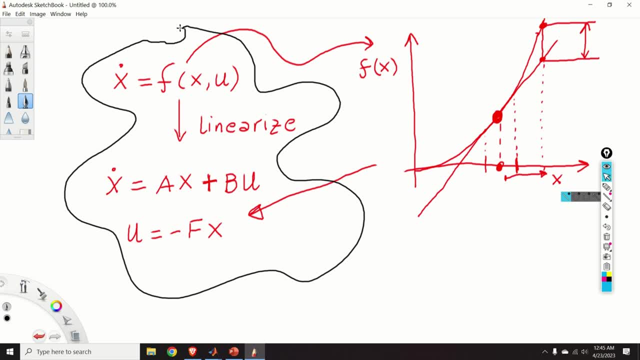 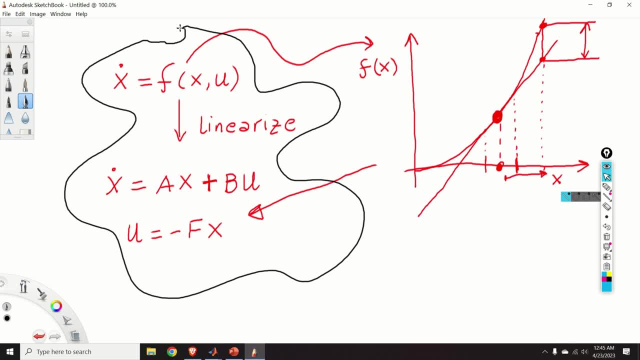 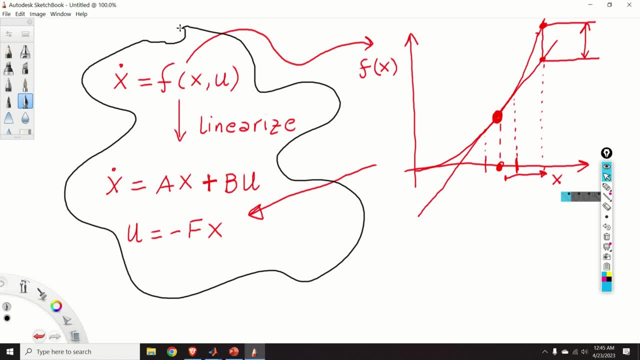 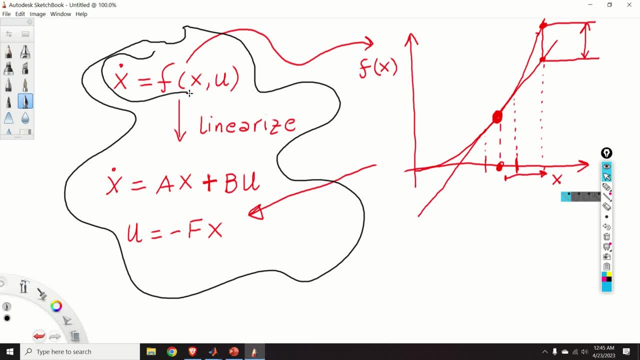 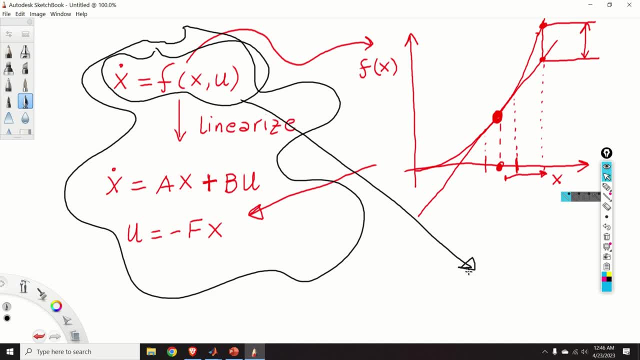 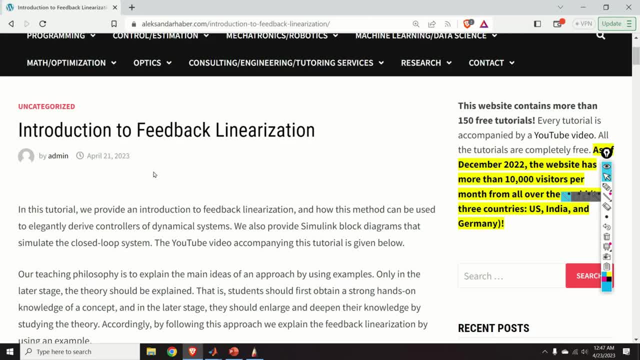 The widely used method is called feedback linearization. Before I start, I would like to mention the following. Those of you who are my subscribers or who follow this channel know by now that I always create a post that nicely summarizes everything that I will explain in this video and, consequently, 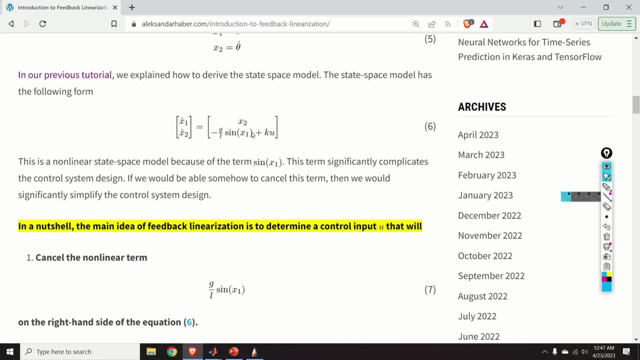 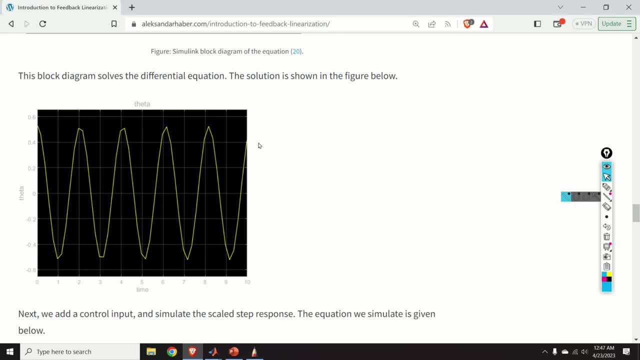 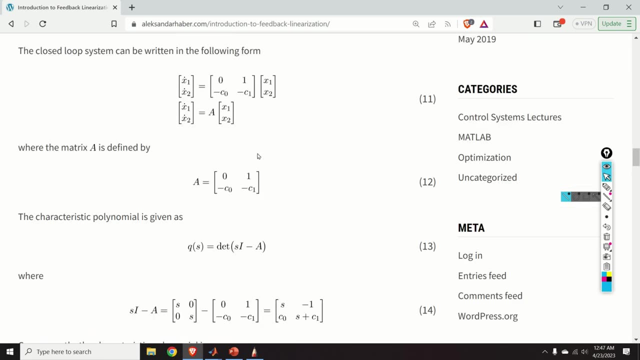 here is the post. This post contains equations, contains all the explanations and it even contains simulink blocks and graphs Which you can find in the description of this video post is given in the description below. secondly, it took me a significant amount of time: energy. 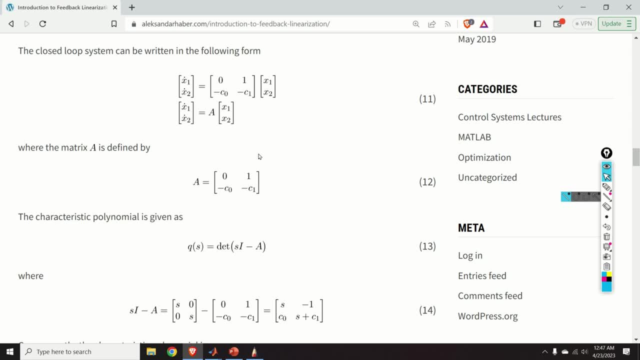 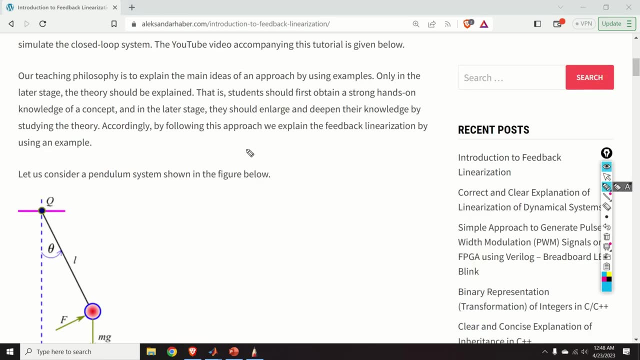 and planning to create this video and this post and consequently, i kindly ask you to press the like and subscribe buttons. thank you, my teaching philosophy is to explain the main ideas of an approach by using examples. only in the later stage the theory should be explained, that is. 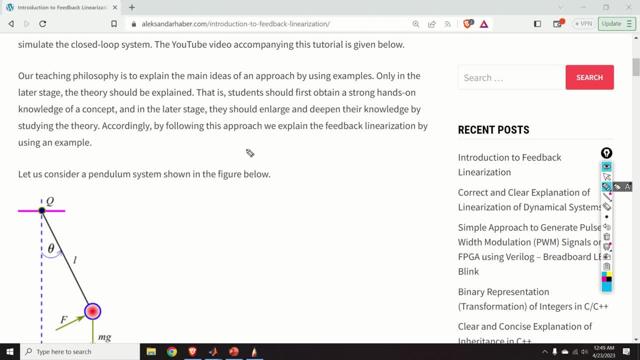 students should first obtain a strong hands-on knowledge of a concept and in the later stage they should enlarge and deepen their knowledge by studying the theory accordingly, by following this approach, i explain the feedback linearization by using an example. so the main purpose of this video is to provide you a quick introduction to feedback linearization by using an example. 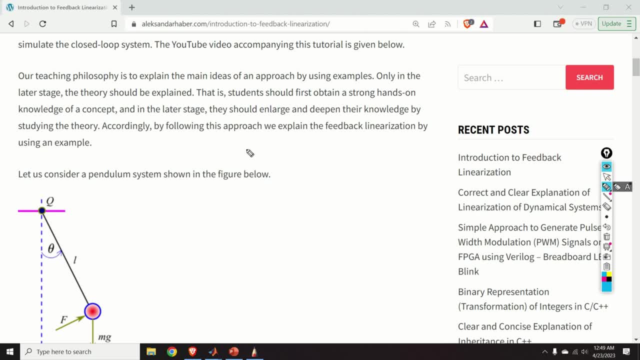 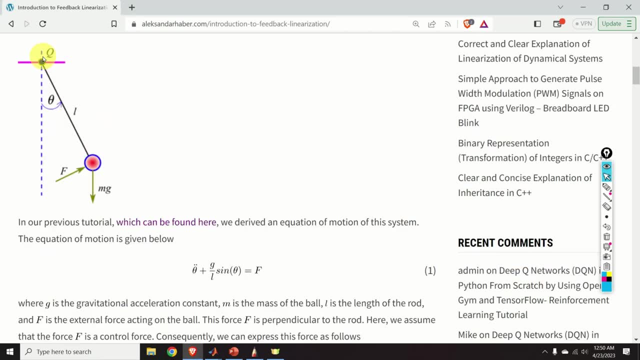 later on you can open the book and you can see how you are going to learn and like and subscribe to the channel and i will see you in the next video, Bye, Bye. to study feedback linearization in more details, Here is the example. 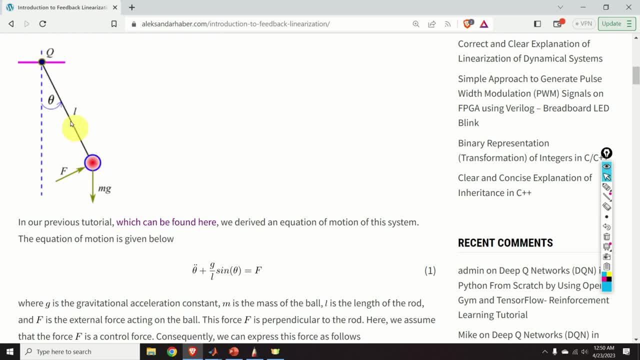 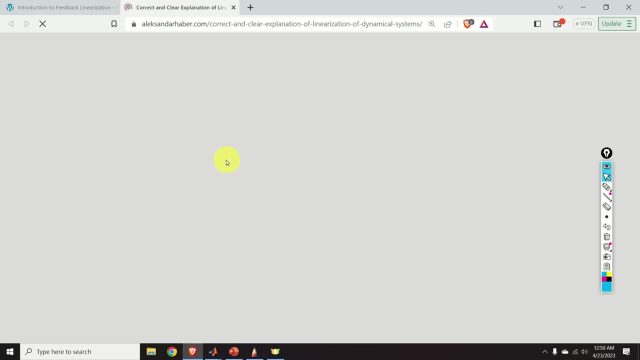 It's a relatively simple system consisting of a ball, a massless rod that's being attached to the ceiling at this point Q. In my previous tutorial, which can be found here, I derived an equation of motion and a state-space model of the pendulum, And here's the 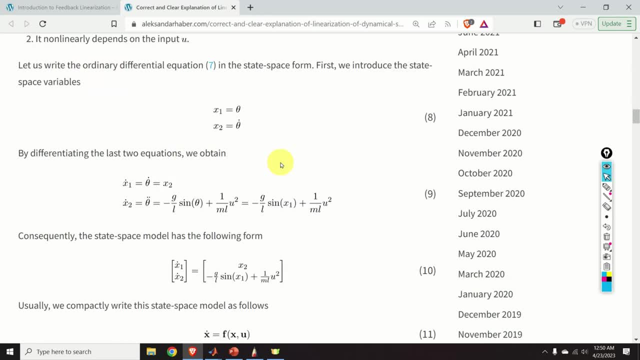 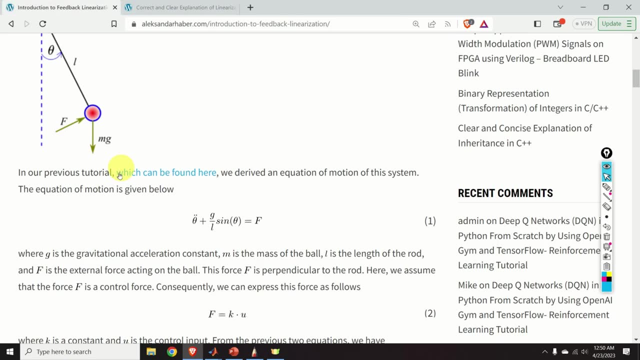 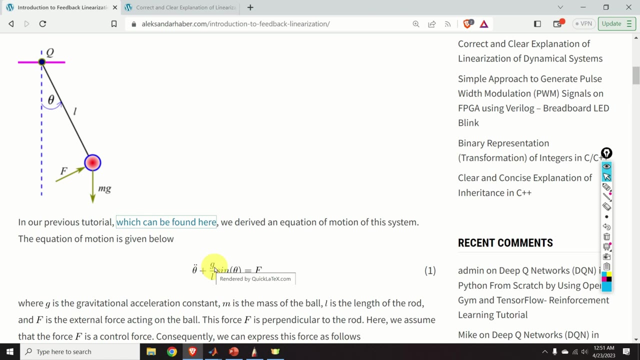 explanation. here's the equation of motion and here's the state-space model. I will use this knowledge and these equations in this video. So here's the equation of motion. Theta is this angle over here. G is the gravitational acceleration constant, L is the. 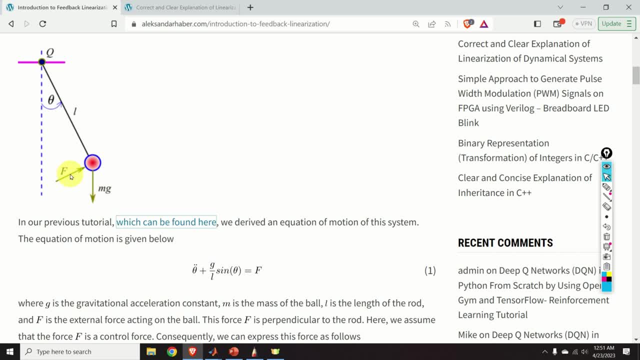 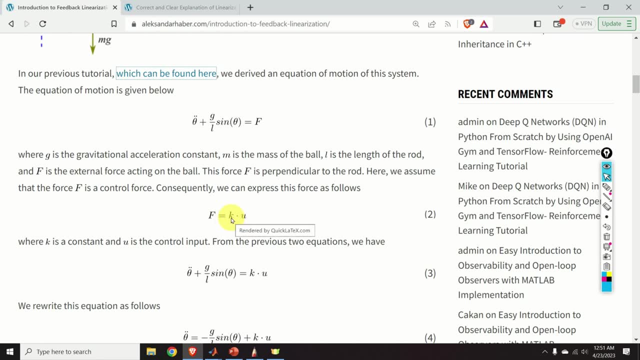 length of the rod and F is the control force. I assume that the control force is equal to K times U, where K is a constant and U is our control input. After substituting this equation in this equation, I obtain the equation that you can see over here. Then we can rewrite this. 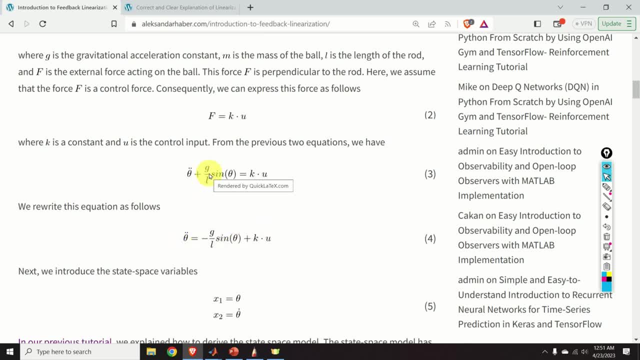 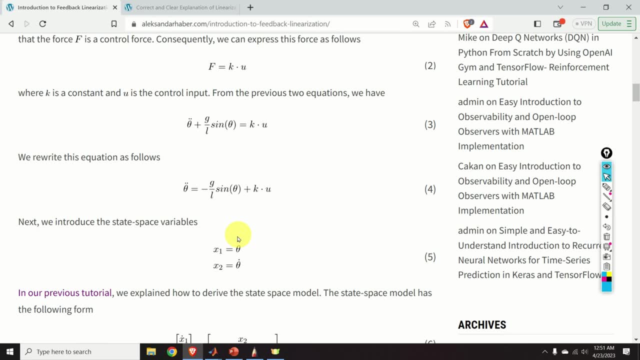 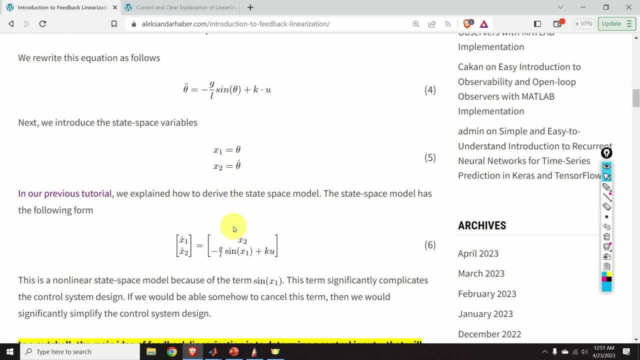 equation like this: We basically take this non-linear term and we put it on the right hand side. Next, let us write a state-space model. We first introduce the state-space variable. X1 is theta, X2 is theta dot. And here is the state-space model. 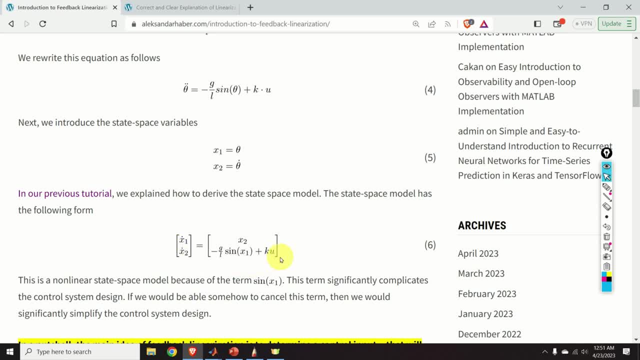 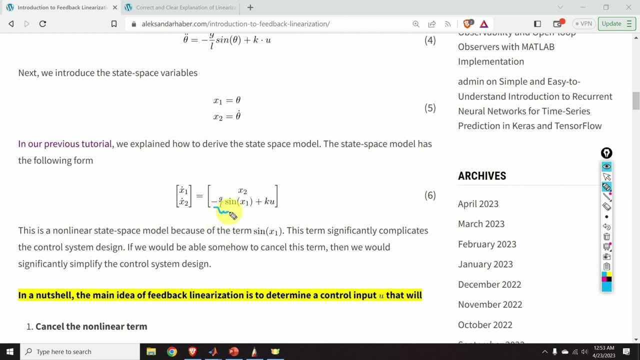 Obviously, this is a non-linear state-space model and the reason is that we have this sinusoidal term on the right hand side. As I mentioned at the beginning of this video, this non-linear term over here significantly complicates control system design. If we would be able to somehow cancel this term. 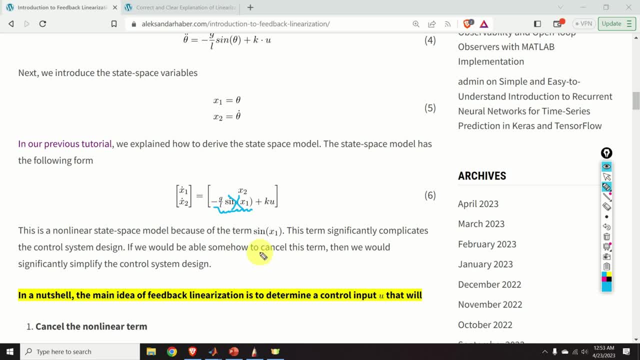 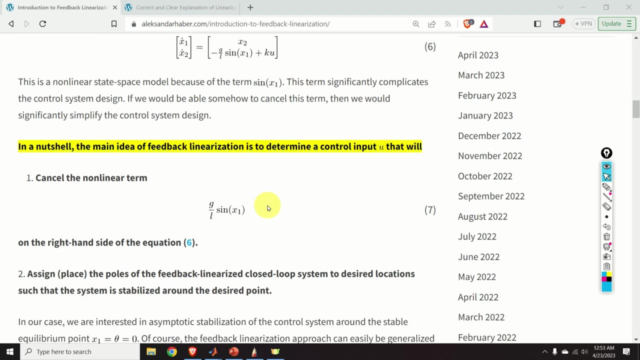 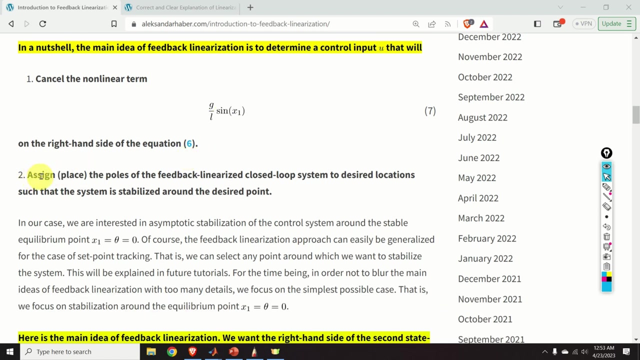 then we would be able to significantly simplify the control system design, And the feedback linearization is actually trying to achieve that. In a nutshell, the main idea of feedback linearization is to cancel this non-linear term and then to find an appropriate form of control input that 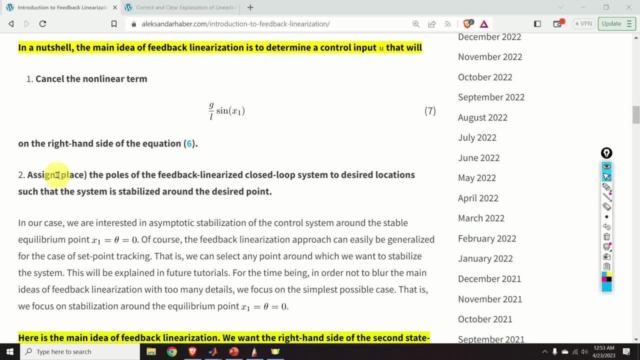 assigns the poles of the feedback linearized closed-loop systems at desired locations, such that the system is stabilized around the desired point. In our case, we are interested in asymptotic stabilization of the control system around the stable equilibrium point that is. X1 is equal to theta is equal to zero And, graphically, 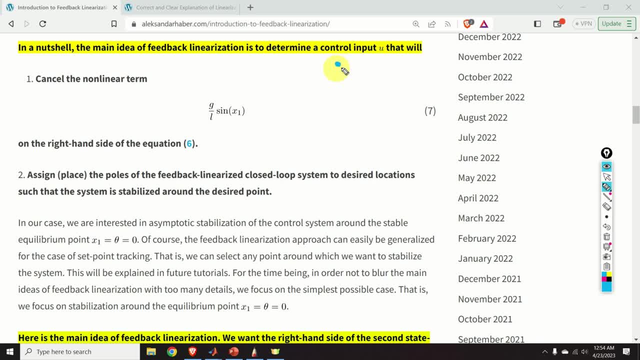 this linearization point is basically this: position over here of the pendulum. This position corresponds to: theta is equal to zero. Of course, the feedback linearization approach can easily be generalized for the case of set-point tracking, For example. we can assume: 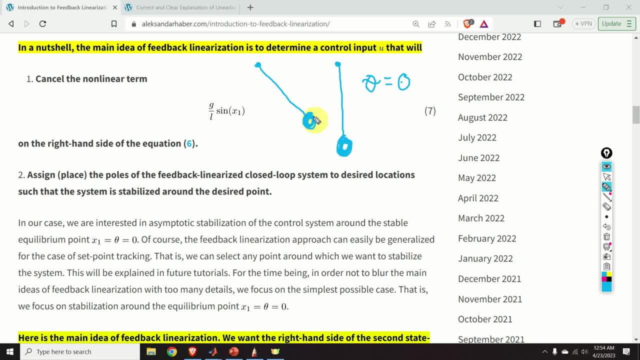 that we want to stabilize our system around this point. let's say theta, where theta is equal to 30 degrees, And this will be explained in future tutorials. For the time being, in order not to blur the main ideas of feedback linearization with too many details, we focus on the 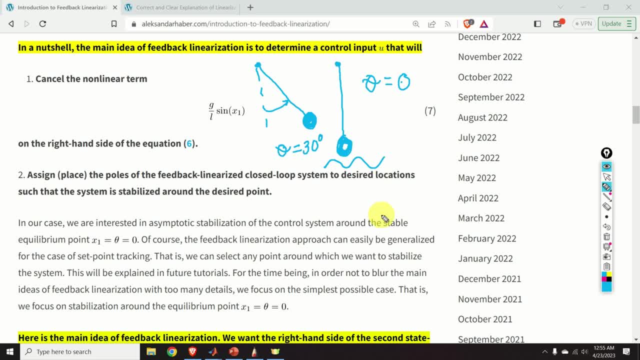 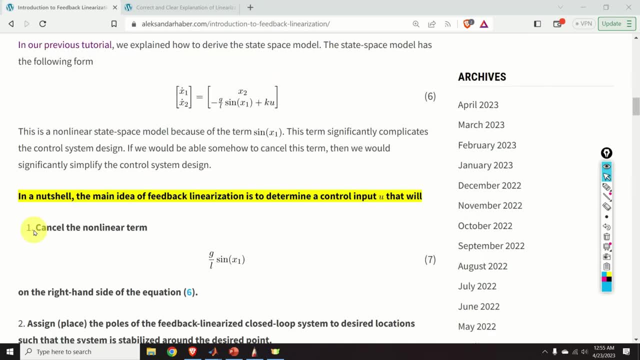 simplest possible case that's illustrated over here, That is, we focus on stabilization around the equilibrium point. X1 is equal to theta is equal to zero. Let us apply the first step of the feedback linearization method. We want to cancel this term. We can. 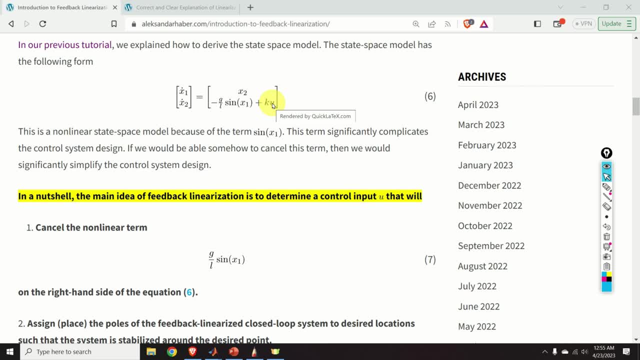 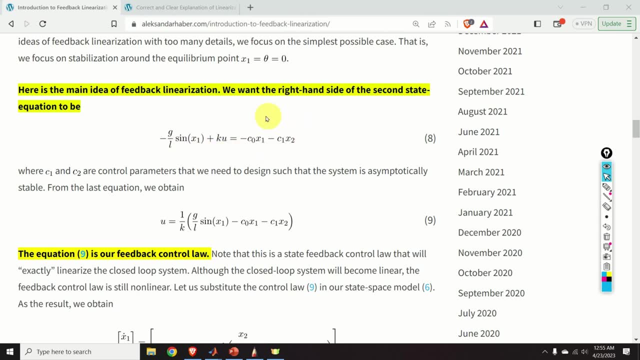 cancel this term by wisely choosing this input u over here. And because we want to cancel the right side of the second state equation, we can simply define this equation So we can say that minus g over L, minus X1, plus k times u should be equal. 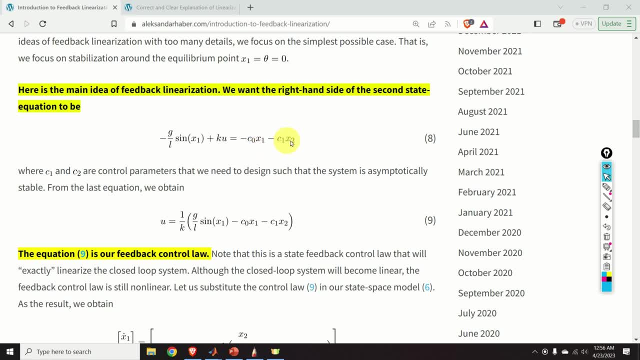 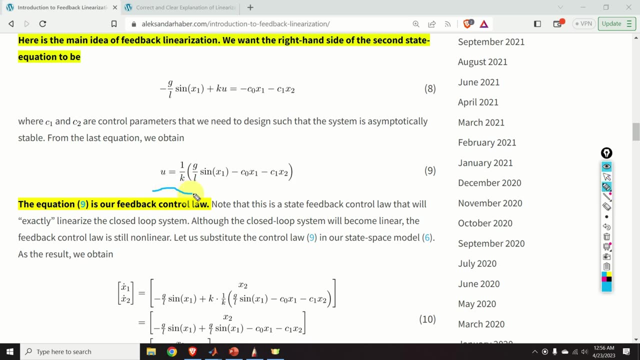 to minus C0, X1 minus C1, X2.. Remember that X1 is theta and C2 and theta dot is equal to X2.. From this equation we obtain our feedback control law that's given over here. Note that this is a state feedback control law that will: 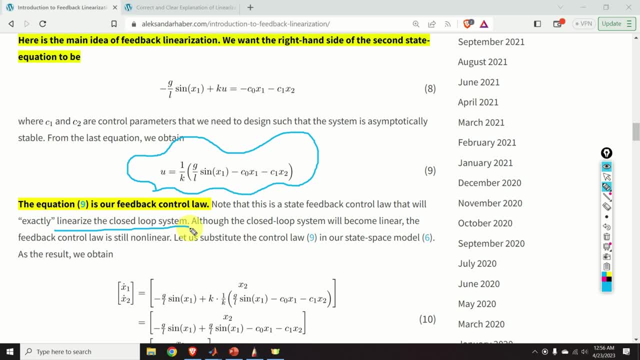 exactly linearize the closed loop system, That is, we are not using Jacobian methods to linearize the control system. This is a very important thing to keep in mind. Another important thing to keep in mind is that, although the closed loop system will become linear, and you will 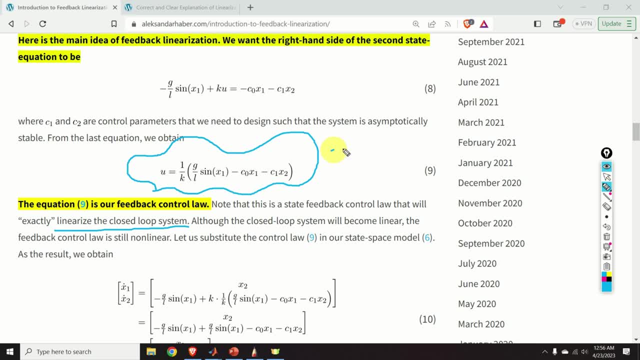 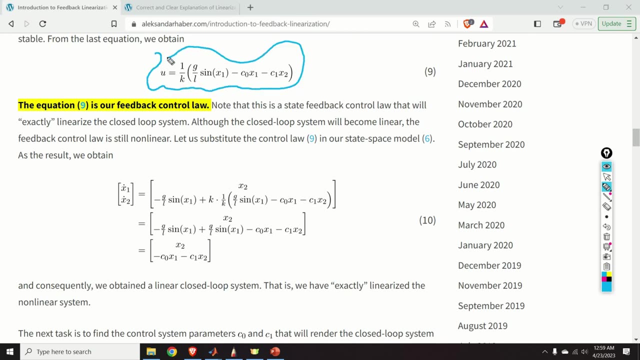 see that in the SQL the feedback control law over here is still non-linear. This is because of this term over here. Next, let us substitute this control law in the second equation of the state space model, And here you can see the result of this substitution. 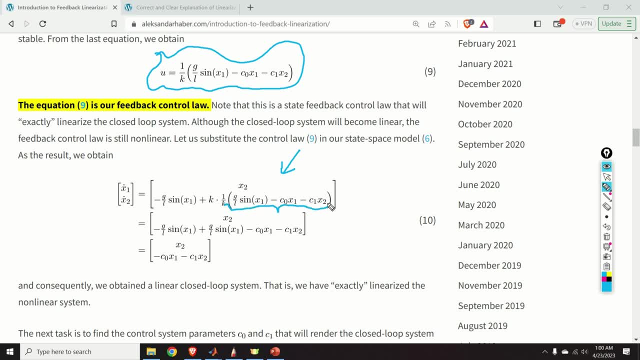 This part over here is our feedback control law that's given over here. Now we can see that k and k can be cancelled and, as the result, we obtain the second expression over here. Then we can cancel these two terms and, as the result, we obtain this equation over here. 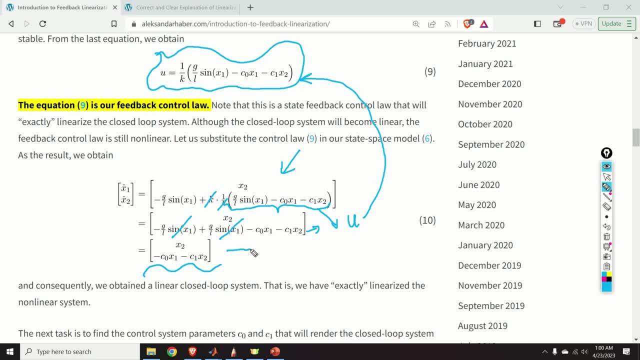 And notice over here that this equation is a linear state space model. To summarize, by applying a non-linear control law to our original non-linear dynamics, we obtained a closed loop system that's completely linear. And that's the magic of the feedback linearization approach: We are able 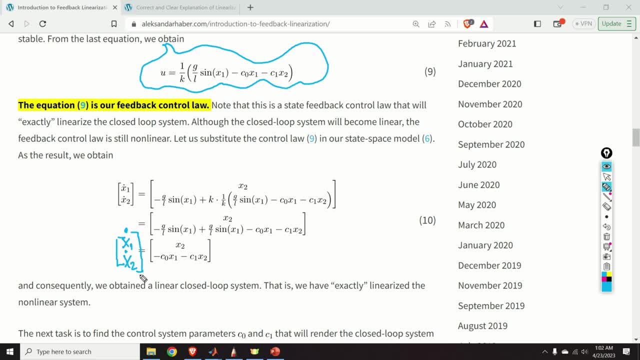 to exactly linearize our closed loop system. The next task is to choose these parameters, c0 and c1, such that the closed loop system is asymptotically stable. By properly choosing c0 and c1, we can make sure that our state, after some time, goes to the equilibrium point. 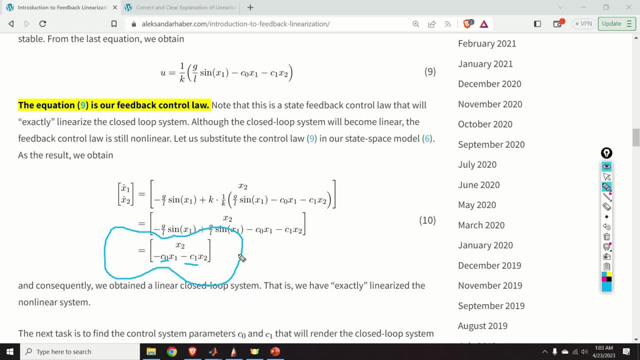 Here I made a mistake by saying: goes to the equilibrium point. since this is a dynamical system and the state trajectory can never reach, in the finite time, the equilibrium point, I need to say the following: The state will reach a very small neighborhood of the equilibrium. 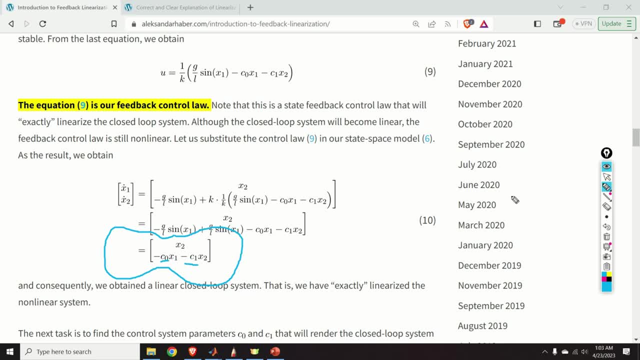 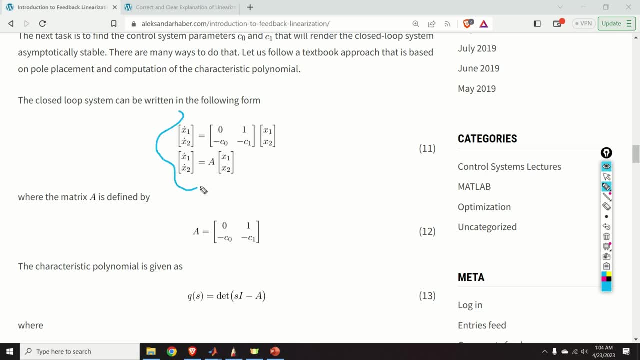 point and that's the correct expression. Okay, so let's see how to find the parameters c0 and c1.. Notice that the last equation can be written in this standard form: where A matrix is given over here, The characteristic polynomial of this system is given over here, That is, it's a determinant. 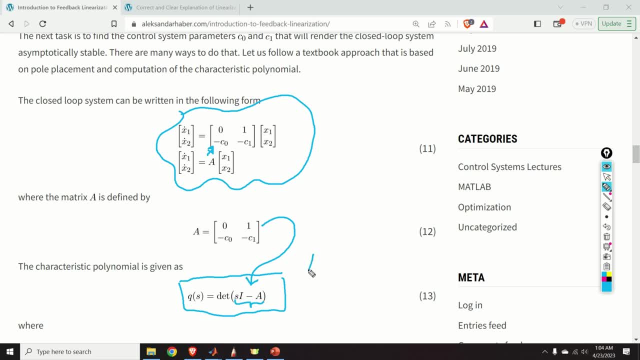 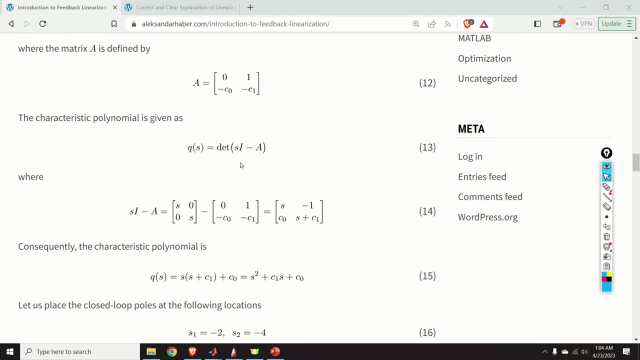 of this matrix given over here, where I is, the identity matrix 1,, 1,, 0,, 0 of diagonals. So let us compute this characteristic polynomial. I can simply write si minus a, and the result is given over here. Then I need: 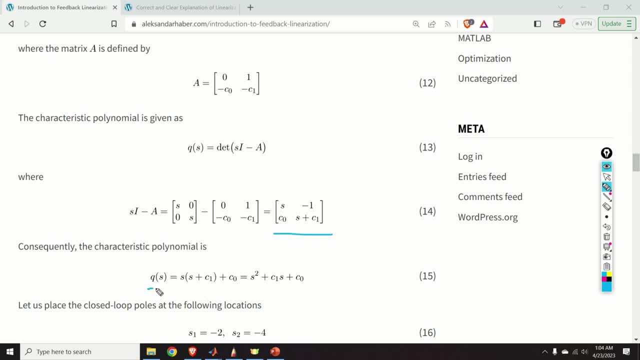 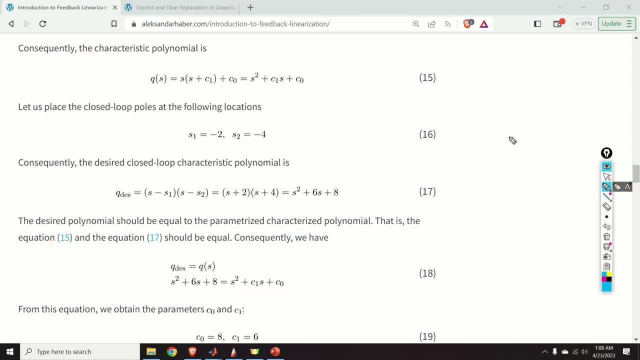 to compute the determinant of this expression, and the determinant is given over here. Basically, the determinant is equal to s times s, c plus 1,- this term over here- minus c0, and that gives plus, and the final expression is given over here. Next, let us use a simple pole placement method to 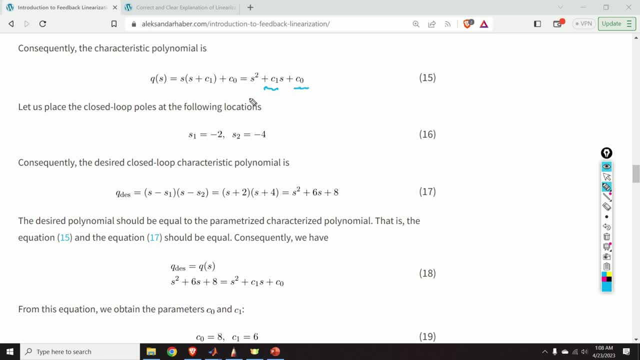 design the parameters c1 and c0.. Let us place the closed-loop poles at the following locations: s1 is equal to minus 2 and s2 is equal to minus 4.. As the result of this pole placement method, the response of the closed-loop system. 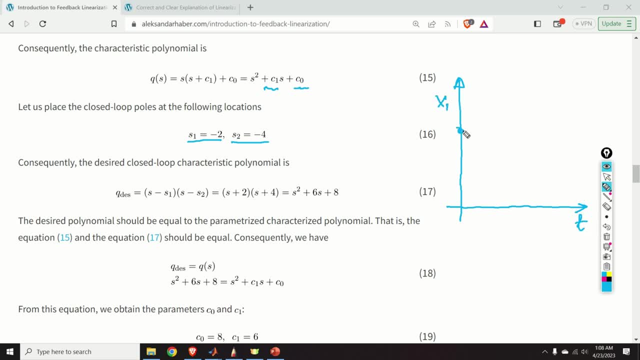 in time should look like this. So both x1 and x2 should decay over time, That is, we will not see oscillations in our response. The desired closed-loop characteristic polynomial corresponding to this selection of the closed-loop poles is given over here. 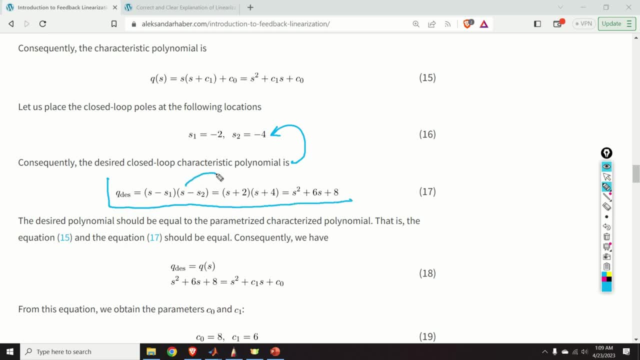 After we multiply this expression, we will obtain s2 plus 6s plus 8.. This desired polynomial should be equal to the parameterized characteristic polynomial. That is, equation 15 and equation 17 should be equal and, as the result, we obtain this equation. 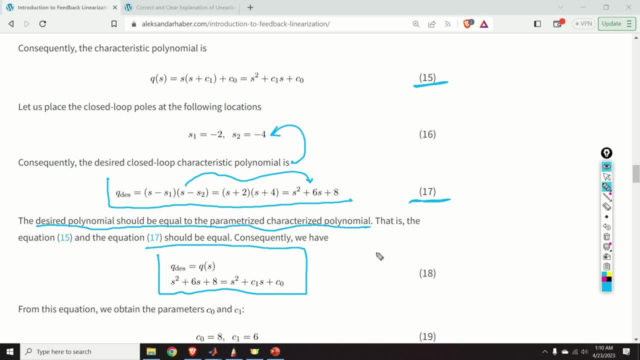 From this equation, we can clearly see that c1 is equal to 6 and c0 is equal to 8.. And this is the final result, That is, these are the parameters that will make the closed-loop system to be asymptotically stable. 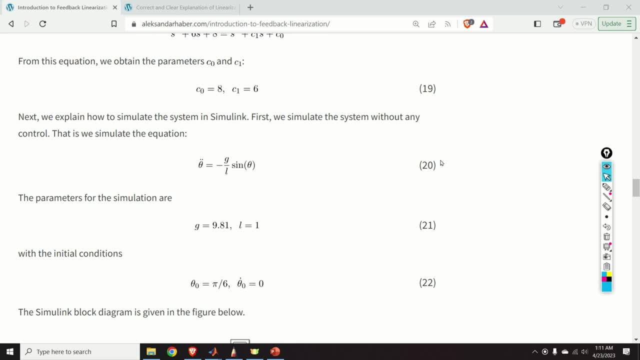 In my next video, I will explain you in detail how to simulate the system in Simulink. However, here, in order to make this video as short as possible, I will only present the results. Let us first simulate the system without any control action. 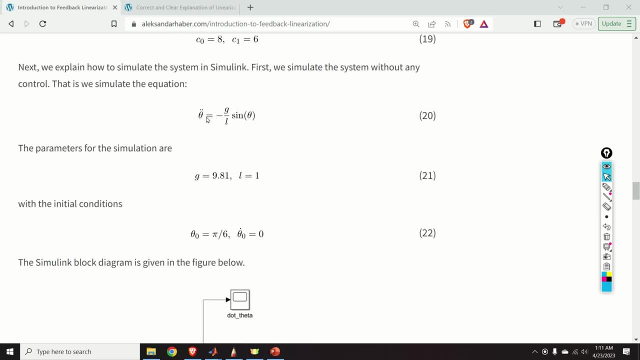 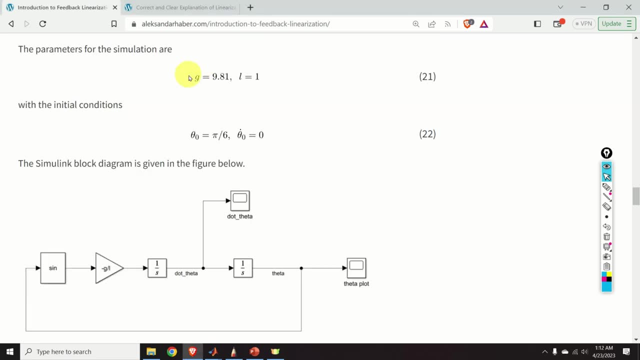 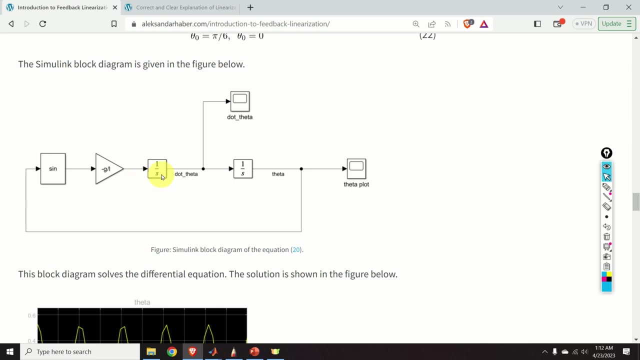 That is, we simulate our equation. θ2 dots is equal to minus g over L sine θ. The parameters used in simulations are given over here And here are the initial conditions. Notice that we have two integrators and here is the nonlinear part of the equation. 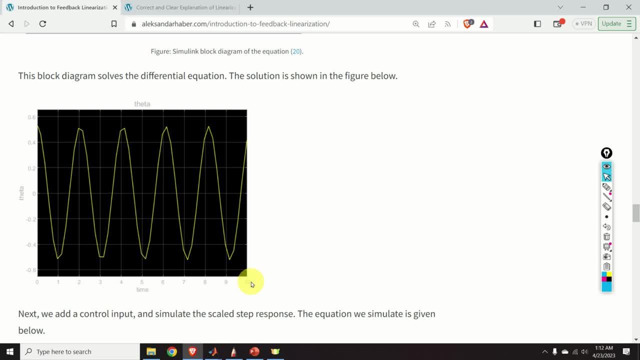 This figure shows the response of the system. Obviously, we will have an oscillatory behavior of θ. This is because the following: If we basically set our initial condition like this, our pendulum will oscillate like this, Where the amplitude of oscillations 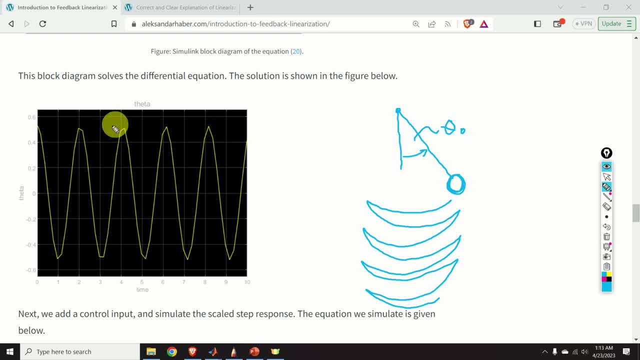 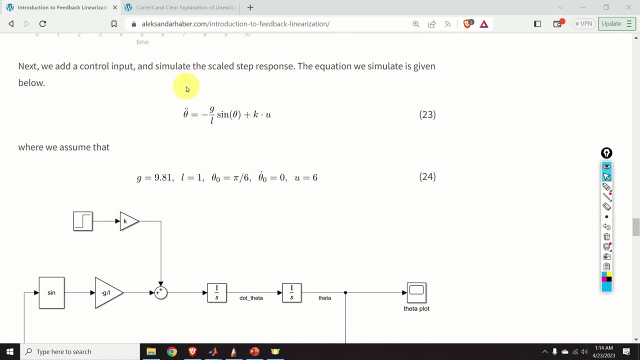 will be equal to θ0.. And this is exactly the amplitude of oscillation, θ0. Next, let us set the control input and simulate the scaled step response. The equation we simulate is given over here, Where the parameters are given here. 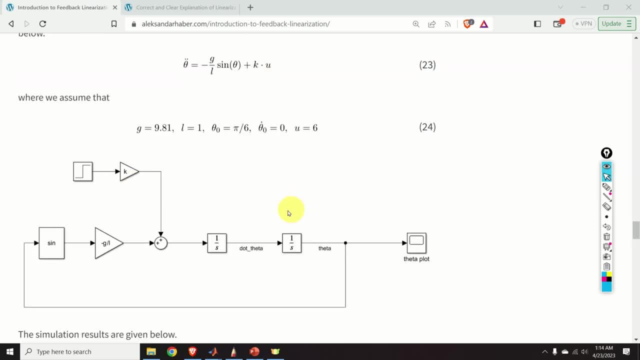 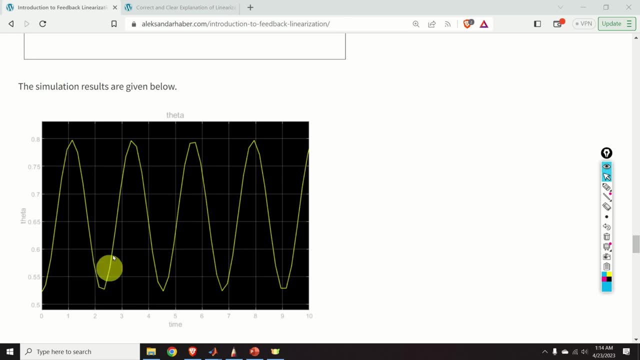 and notice here. here is the block diagram of such a system in Simulink And when we simulate this system we obtain this response Over here. you can observe that this control input biases our response, That is, it shifts the response vertically. 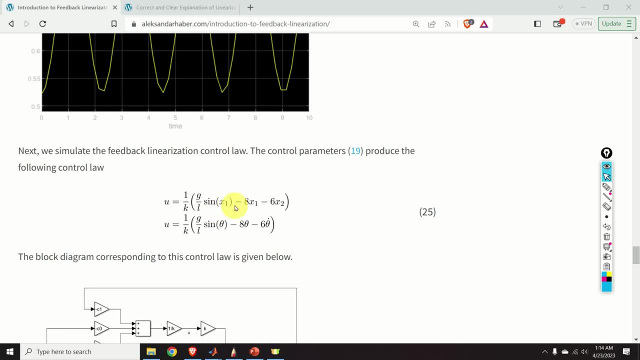 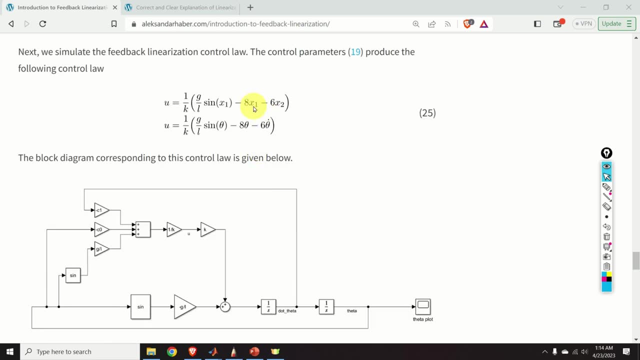 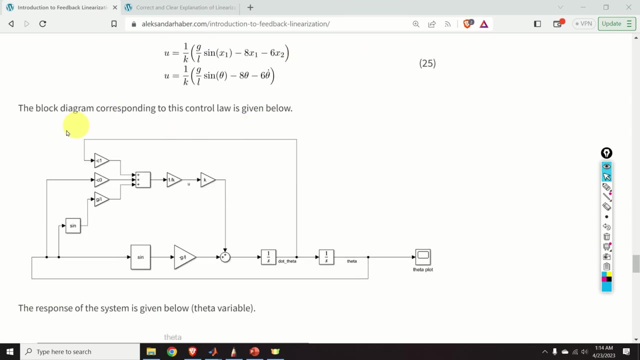 Next we simulate the feedback linearization control law. We substitute c1 and c0 and instead of x1 we can write θ, and instead of x2 we can write θ. And here is the block diagram in Simulink that simulates: 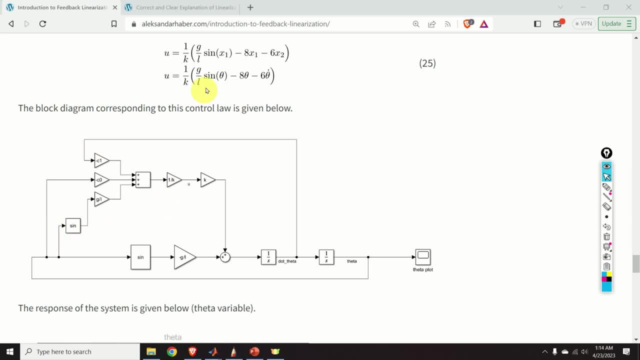 the feedback linearization law. Here is our feedback law. Notice how I created this law. I took θ. I applied this θ to sinus block. This is sinus θ. then I multiplied this term by g over L and I obtained that I have the second term.